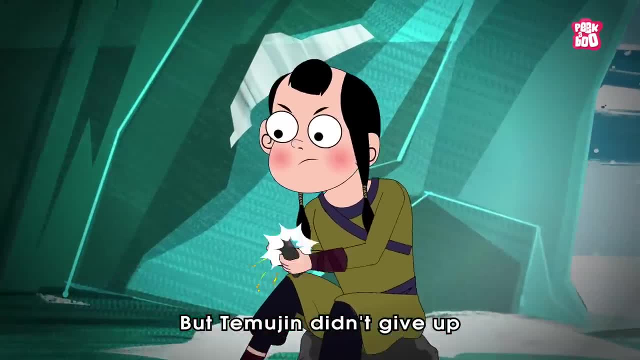 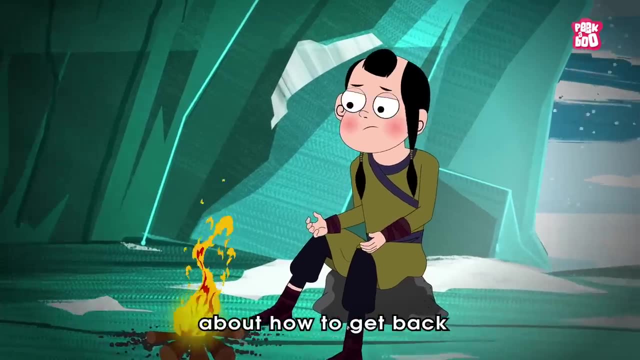 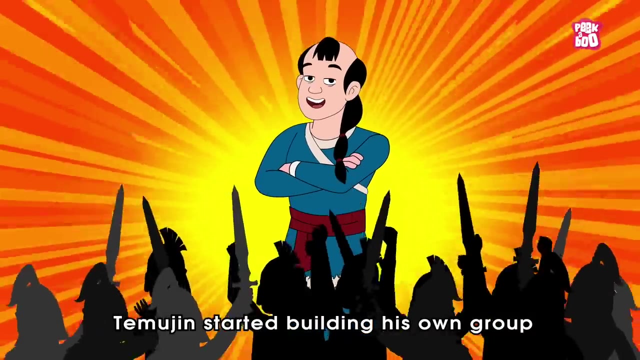 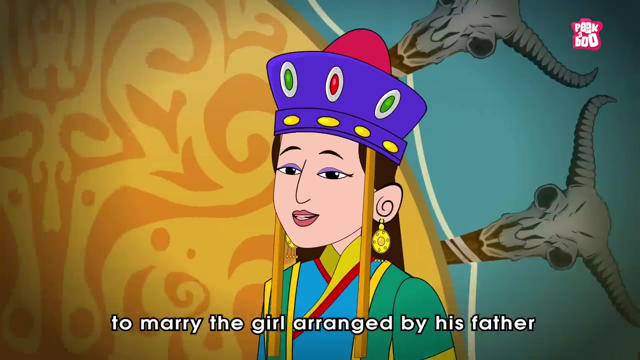 But Temujin didn't give up and made sure his family survived the icy winter, And then he started thinking about how to get back at the Tatars for hurting his dad. So in the coming years Temujin started building his own group and visited the powerful Ongirath tribe to marry the girl arranged by his father and teamed up with her tribe to make his group stronger. 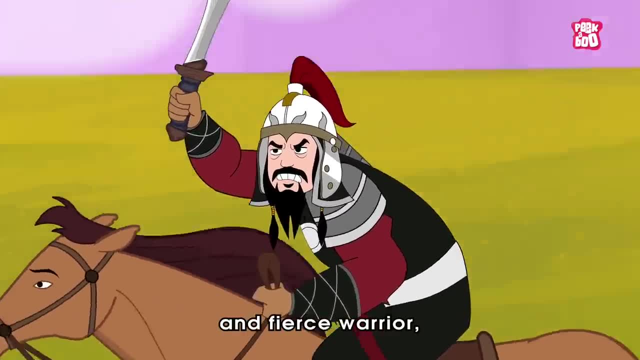 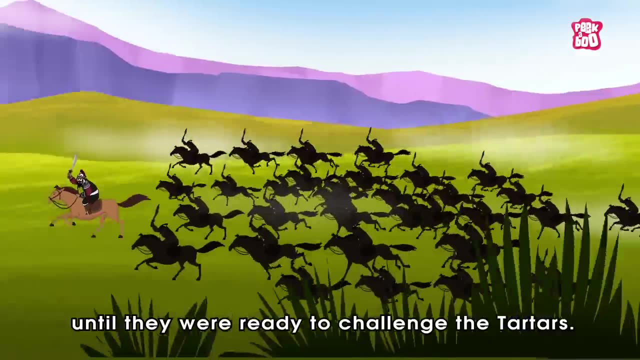 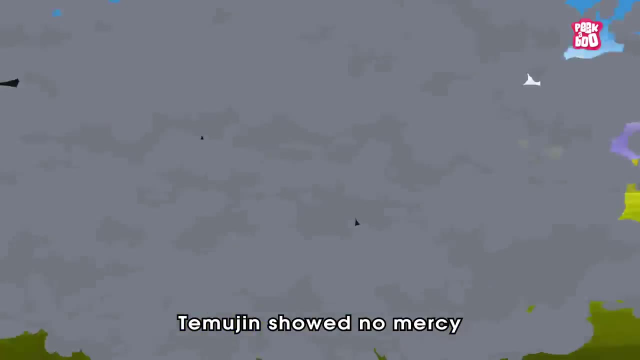 After this, Temujin evolved into a determined and fierce warrior, as his group of warriors continued to grow, becoming larger and stronger, until they were ready to challenge the Tatars. When the battle finally occurred, Temujin showed no mercy and defeated the rivals. 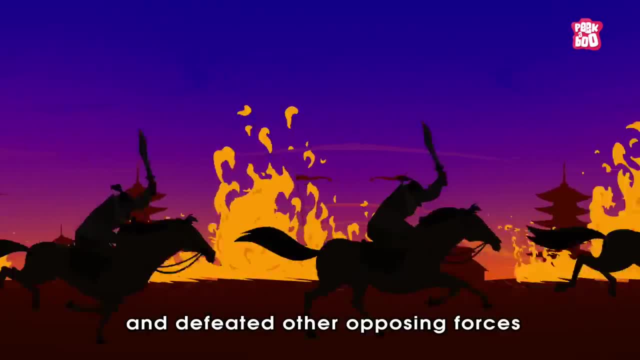 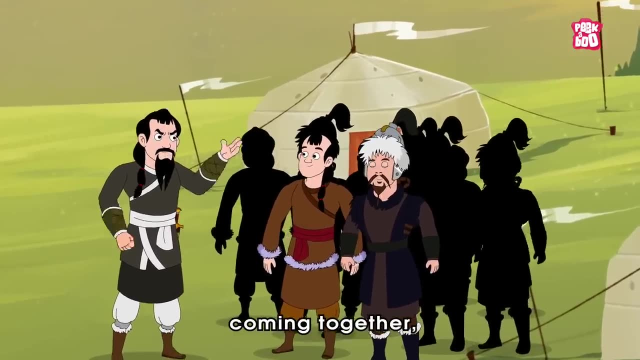 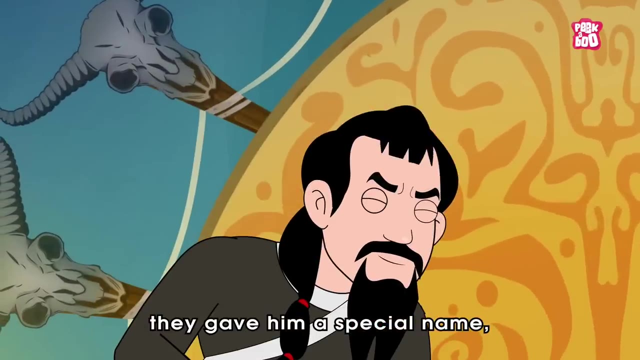 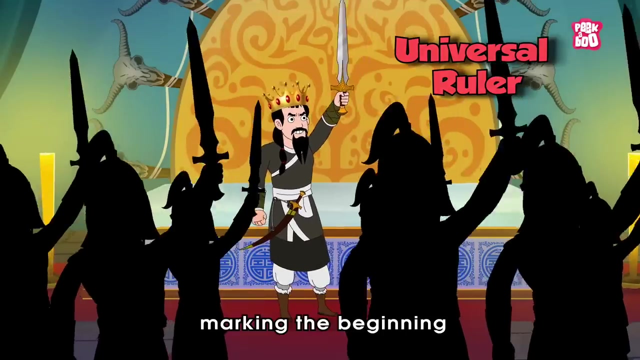 Later on, he continued his conquest and defeated other opposing forces, But made them understand the importance of all Mongols coming together. as they agreed to follow him And in 1206, they gave him a special name, Chinggis Khan, which means universal ruler, marking the beginning of a unified Mongol force. 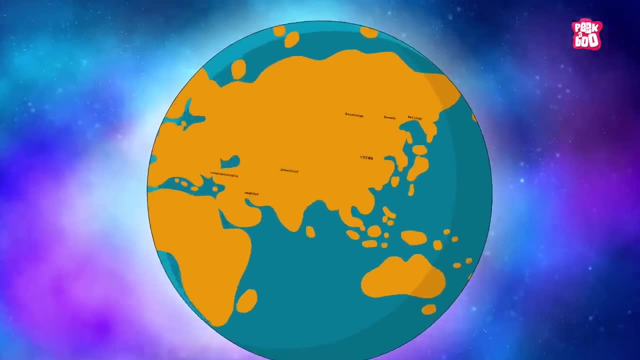 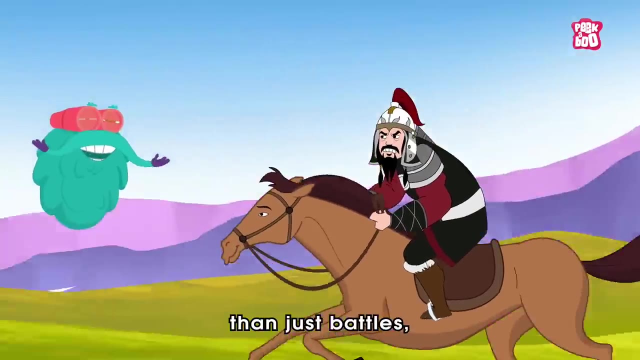 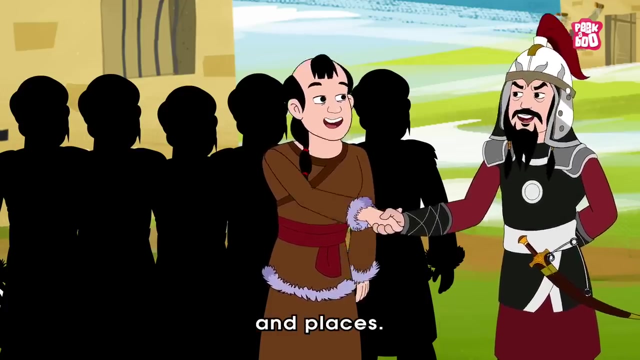 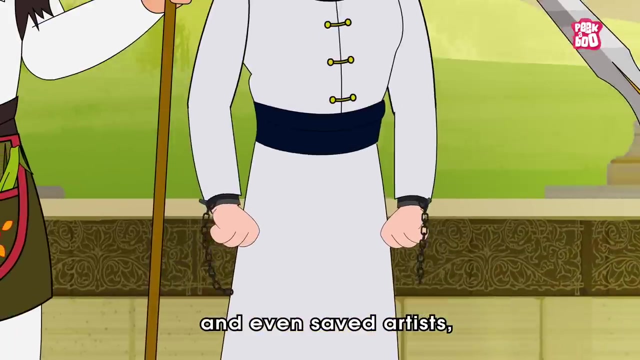 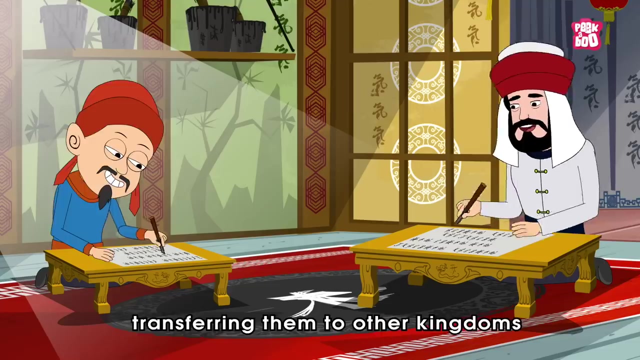 Under his leadership, the Mongols first conquered most of China and the eastern Islamic territories. But his impact was far greater than just battles, as he saw beyond fighting and believed in connecting people and places. His empire practiced religious tolerance among all subjects and even saved artists, doctors and other scholars from conquered places, transferring them to other kingdoms to spread knowledge. 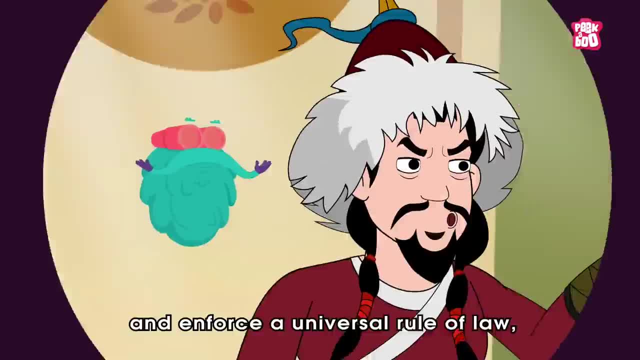 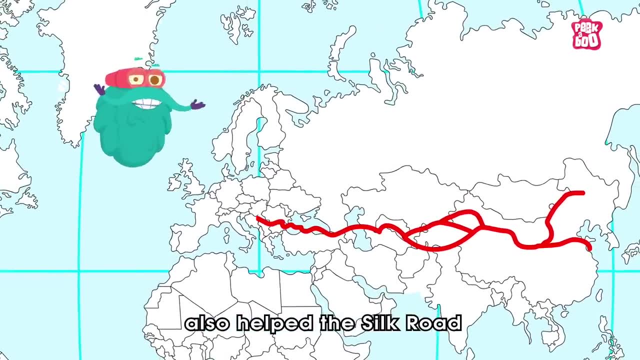 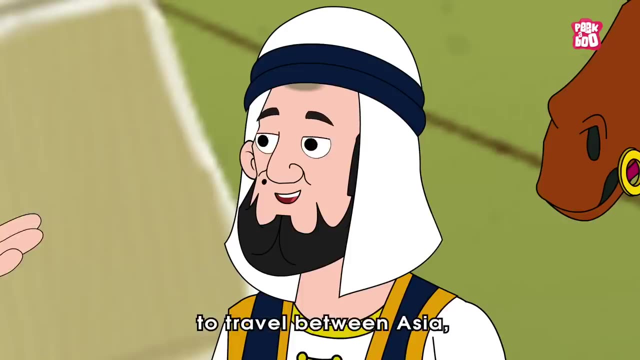 Not only did they establish a vast postal system and enforce a universal rule of law, but the expansion of the Mongol Empire also helped the Silk Road flourish again. This allowed for the exchange of trade, ideas and cultures to travel between Asia, the Middle East and Europe.